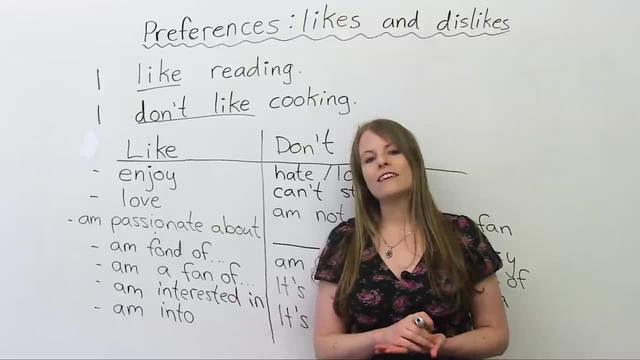 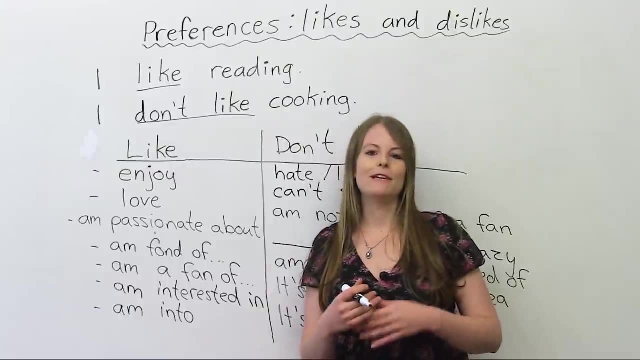 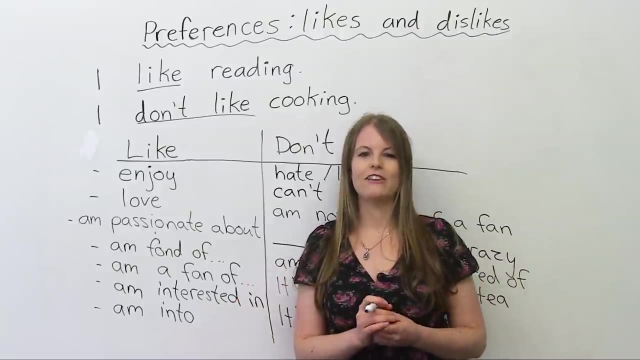 really do not like In my life. I want you to think about something you like and something you don't like. Maybe you like movies, Maybe you don't like winter or cold. Okay, So think about one thing you like and one thing you don't like. Okay, Once you have that in your mind, I want you to 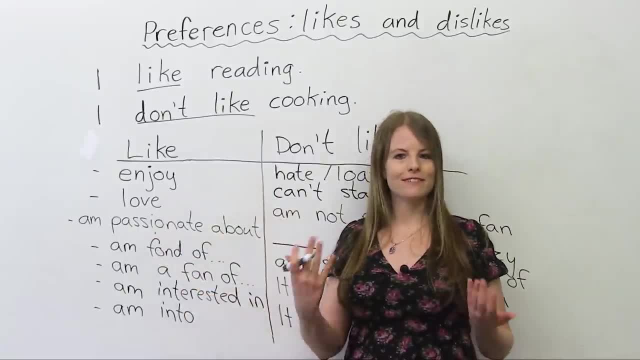 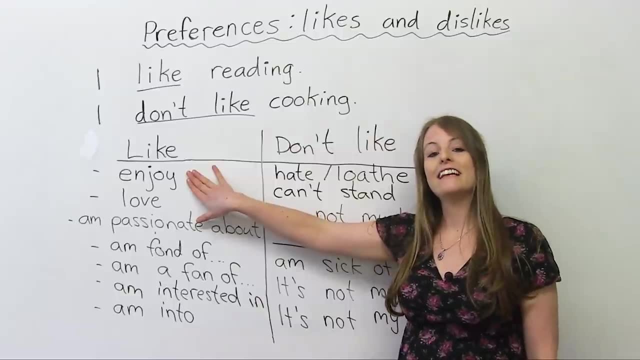 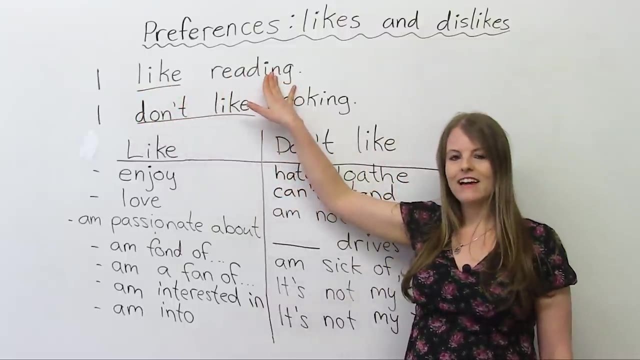 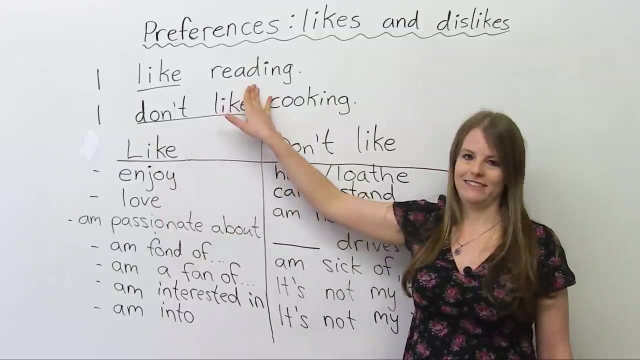 follow me as I teach you some words to describe your feelings. Okay, So the first word we can use when we talk about like is enjoy, For example. I enjoy reading, I enjoy movies, I enjoy shopping. I love reading, I am passionate about reading. 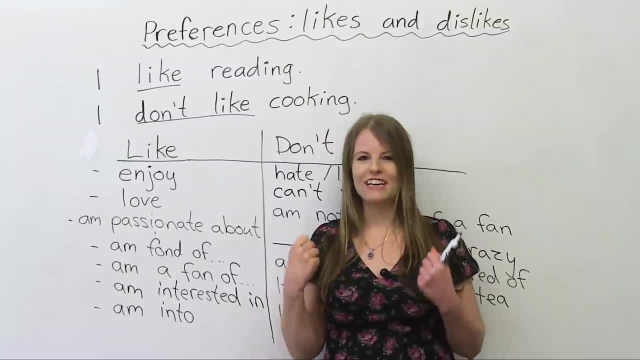 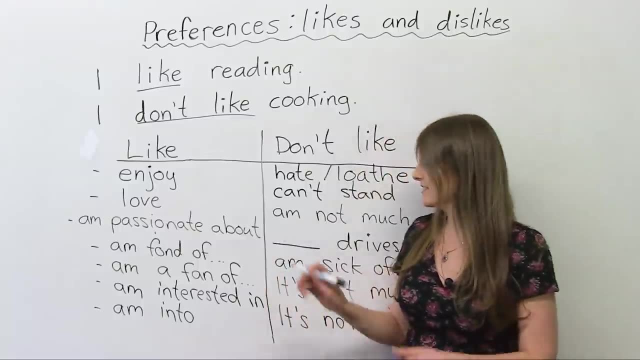 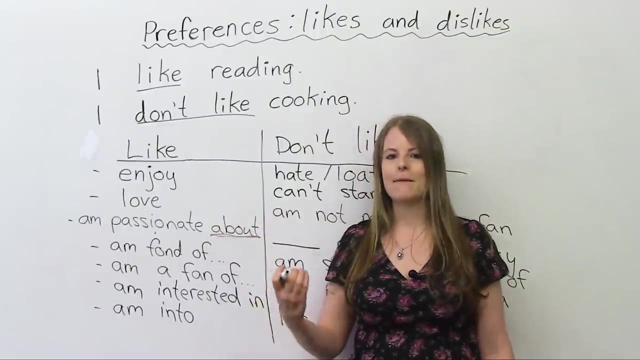 For this one. it means very strong, like You really really like something. You really really enjoy reading. You are passionate about reading, Okay, And I do really like reading a lot, so I would use this. Please pay attention to the preposition that goes with this. I am passionate about something. 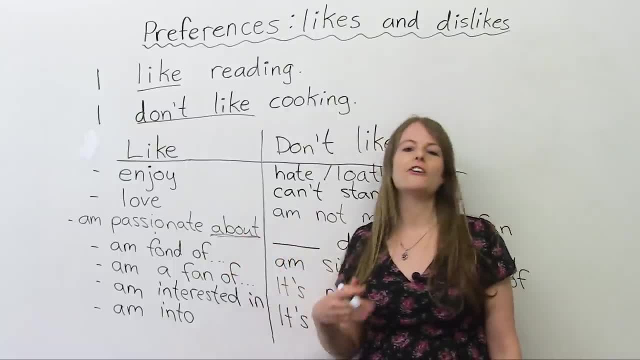 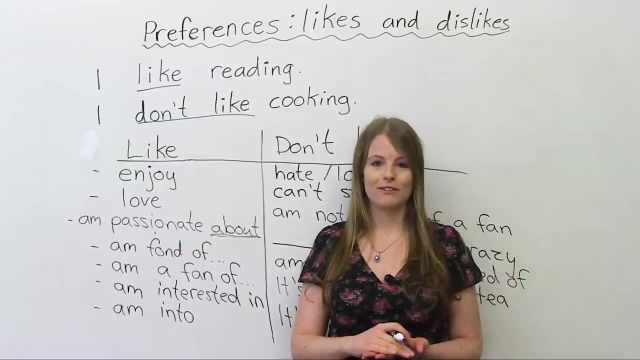 Are you passionate about music? Are you passionate about Justin Bieber? Or maybe you're passionate about the Beatles or Taylor Swift. Maybe you don't like them at all, But think about them. like these three words, you need to add a blank. Well, if you add blank letters to each of the three words, is this a blank? Most likely, not editing your answer is a big deal with historically neglected folks. Thank you for your supportك. 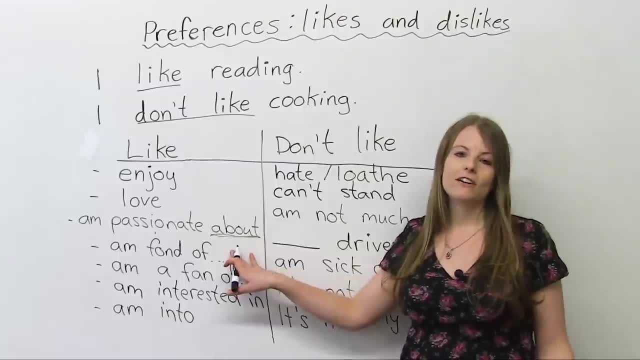 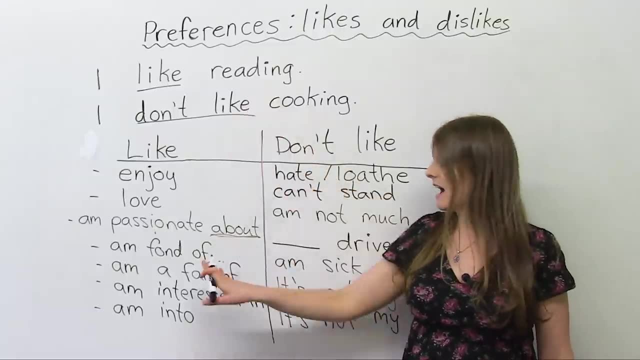 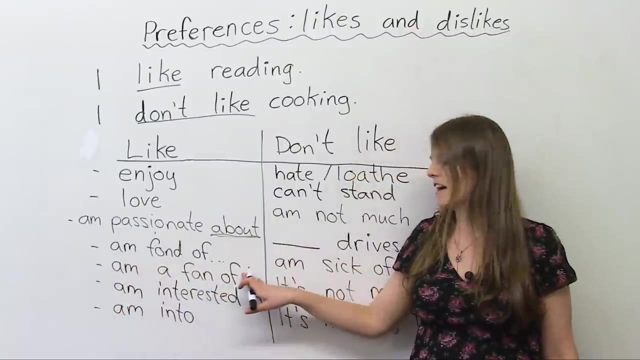 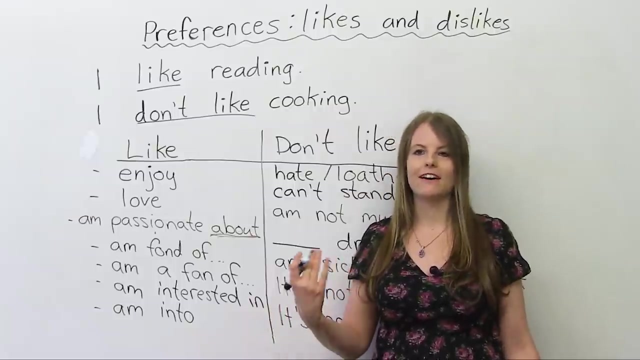 Think about something you're passionate about. We can also use the word I am fond of reading. I am fond of reading. Similarly, I am a fan of reading. I am a fan of hockey, I am a fan of soccer, I am a fan of baseball. 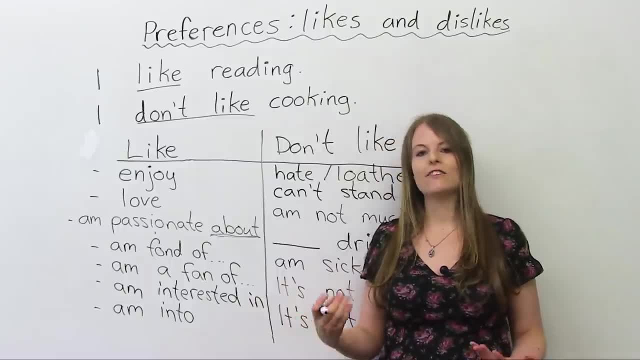 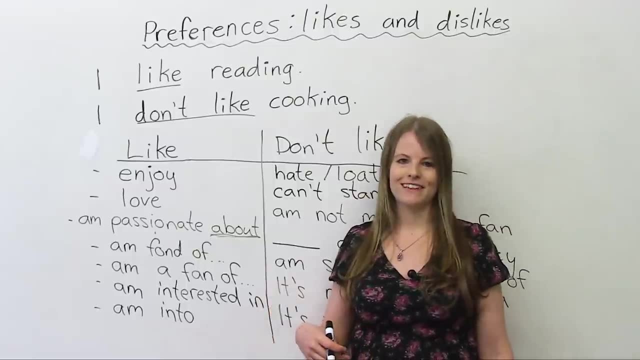 I am a fan of Canada. Okay, So again, this means you really like something I am interested in. I am interested in shopping. If you like a guy or a girl, you can also use this too for someone you have a crush. 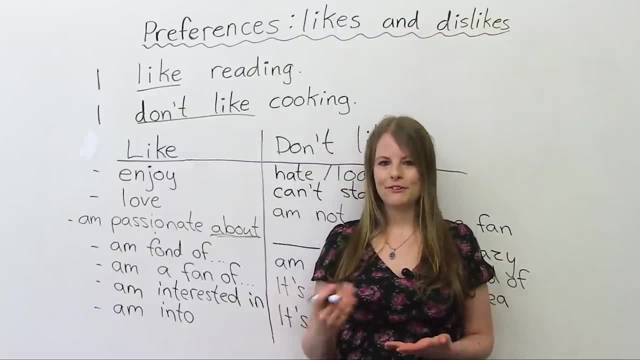 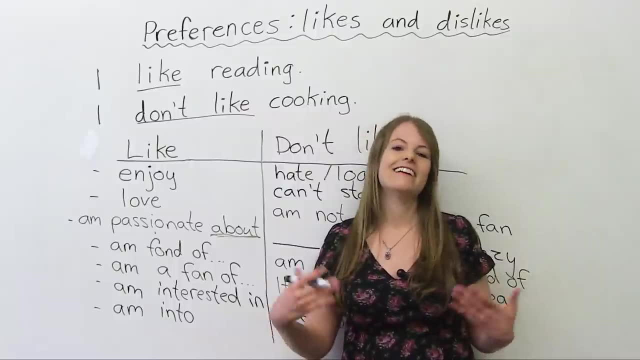 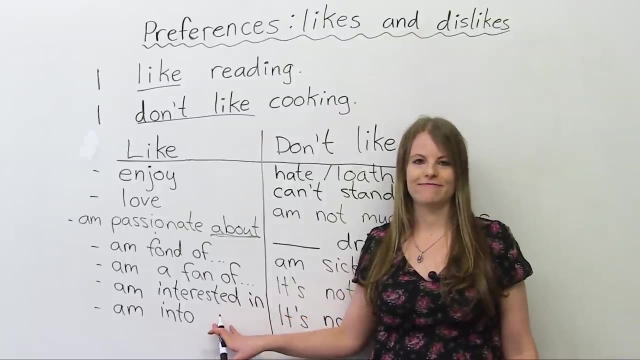 on. I'm interested in Brad Pitt. I'm interested in- Well, not Justin Bieber, but I can't think of any other names. I'm interested in Bob, example. I am into, I'm into scuba diving, I'm into travelling. 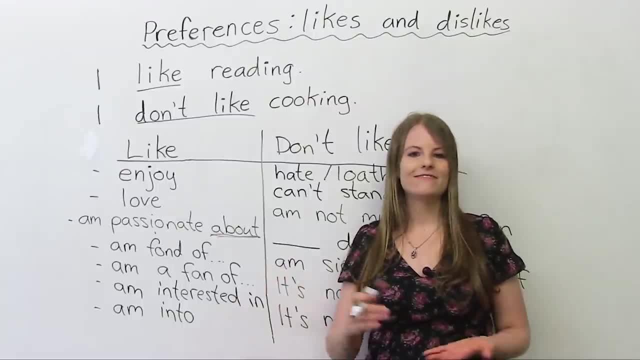 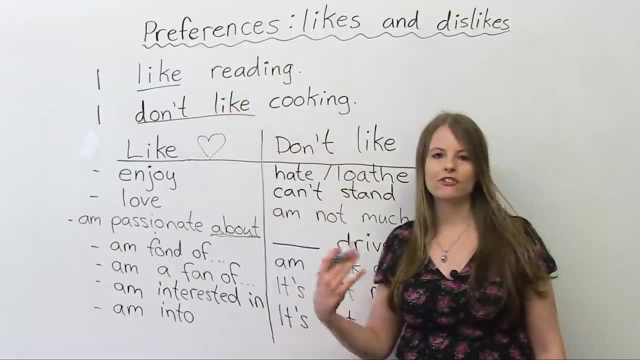 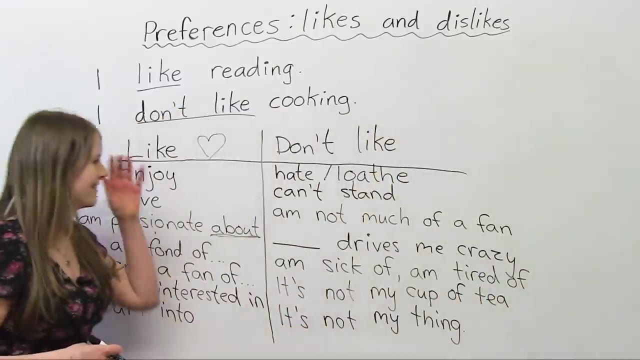 I'm into going to the beach, Okay. So again, all of these mean the same thing pretty much as like or love. So now let's look at some words that have the opposite meaning. Don't like, Okay. And like I told you before, I don't like cooking. 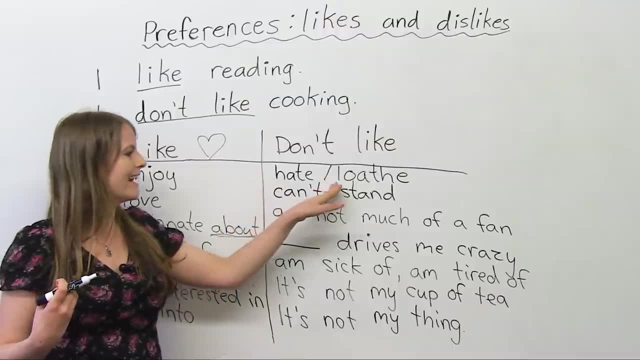 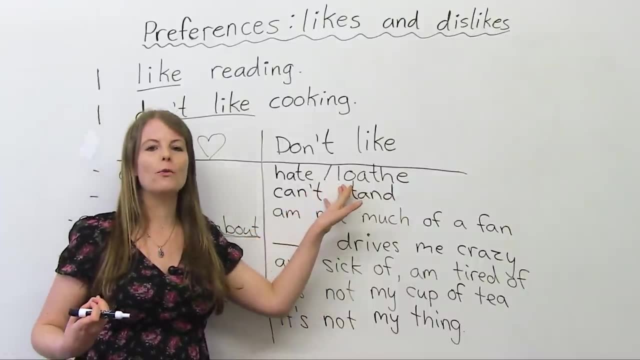 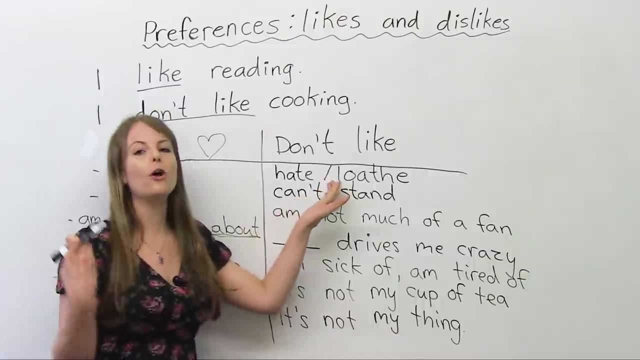 I hate cooking. Okay, Now, if you want to sound like an academic, at an academic level, we also have this word loathe, and it means hate like a lot. You really really hate something. you loathe it, Not love it- loathe. 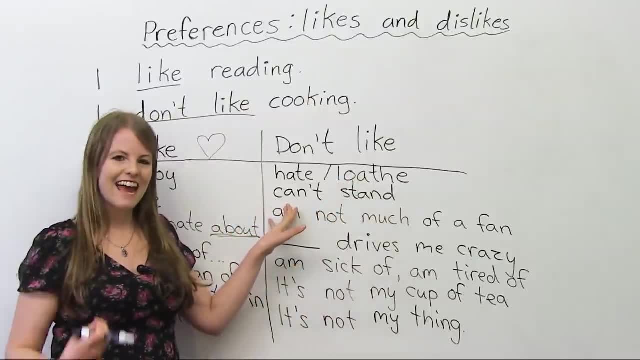 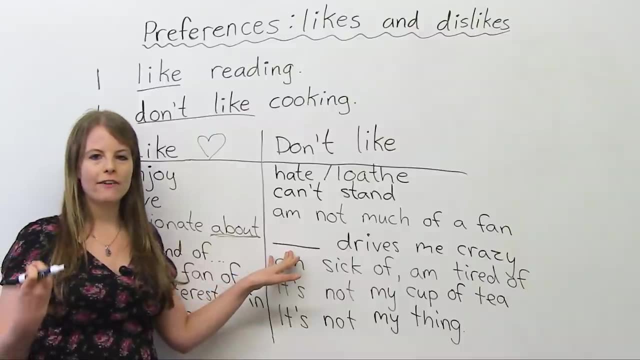 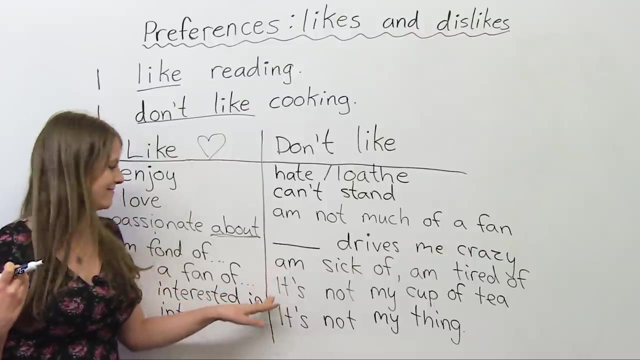 Okay, You can't stand it. I can't stand cooking. I am not much of a fan of cooking, Cooking, Cooking- It drives me crazy. I am sick of cooking. I am tired of cooking. Cooking is not my cup of tea. 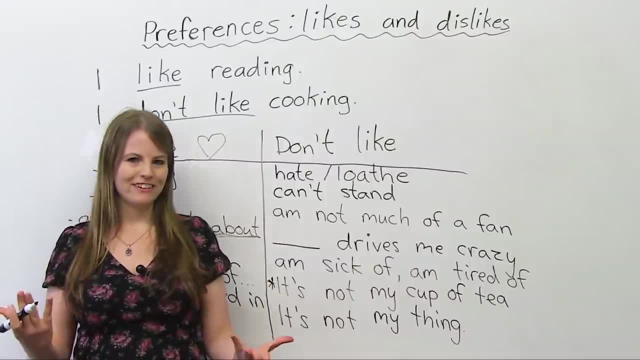 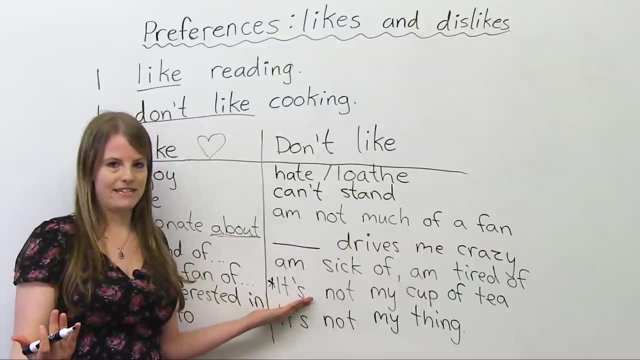 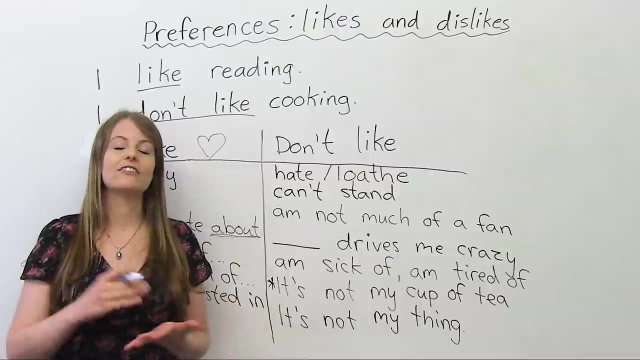 So this one, actually, I really like- It's a very strange expression- not my cup of tea and it means you don't like something. Justin Bieber is not my cup of tea. You know certain types of food. They're not my cup of tea. 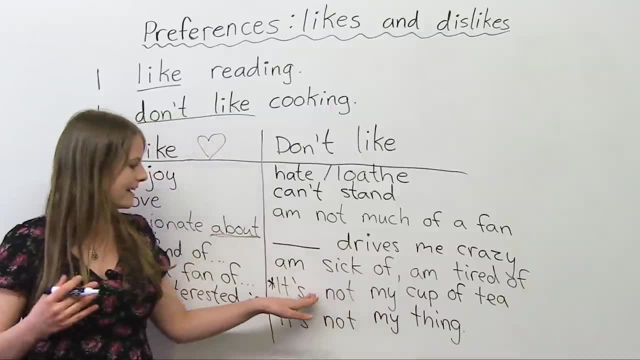 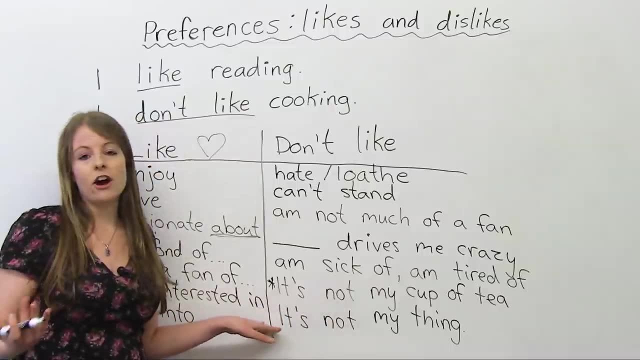 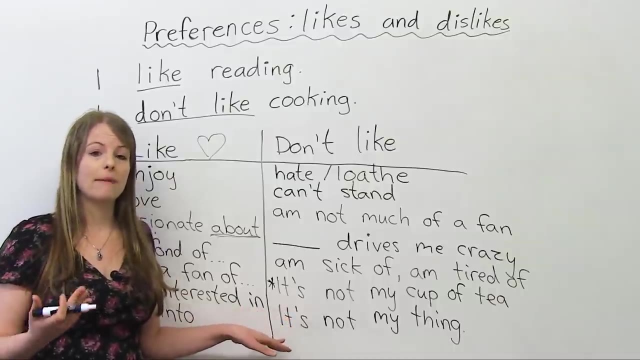 Okay, Not my cup of tea. And again, this has nothing to do with tea. It actually just means you don't like something. You can also say: it's not my thing, Cooking is not my thing, Playing video games is not my thing. 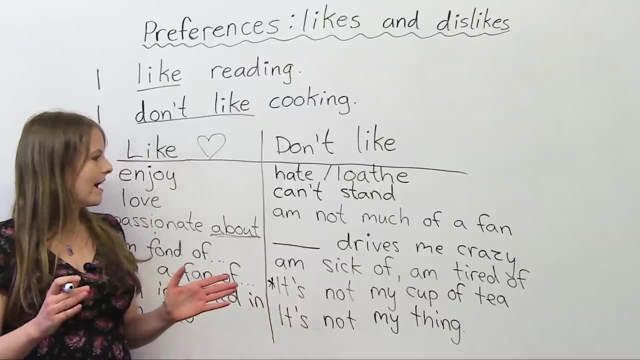 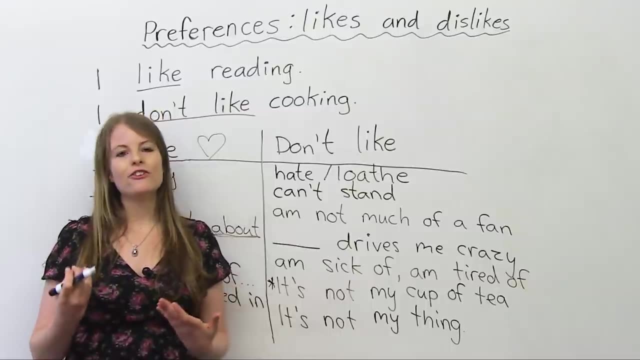 Okay, So just some examples here. So when you're speaking to your friends, When you're talking, maybe in class, I want you to try to use some of these words, just so you're not always saying I like, I don't like. 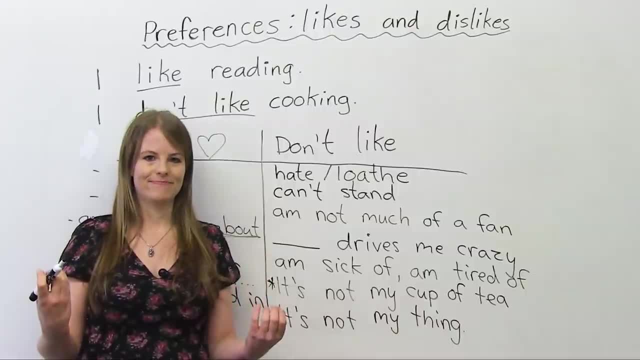 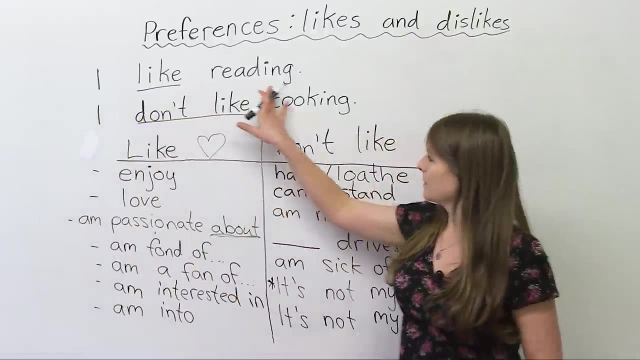 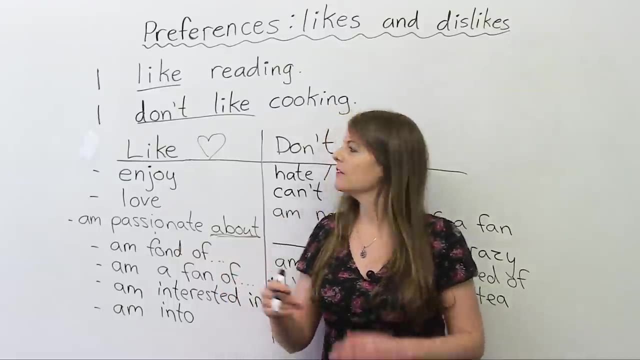 These will make your vocabulary a lot more interesting. Now, there's one other thing I wanted to tell you about these words, and that's looking at my example here. When you have two verbs in a sentence, When you have verb one, Verb two,